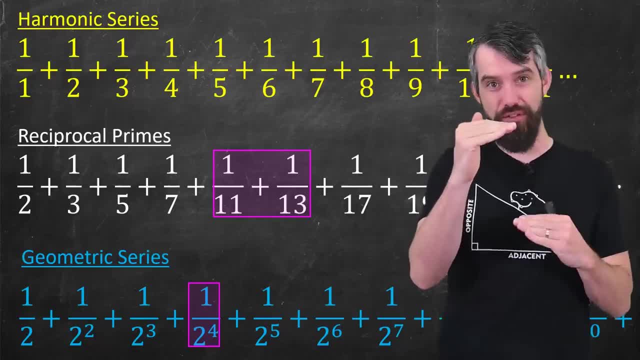 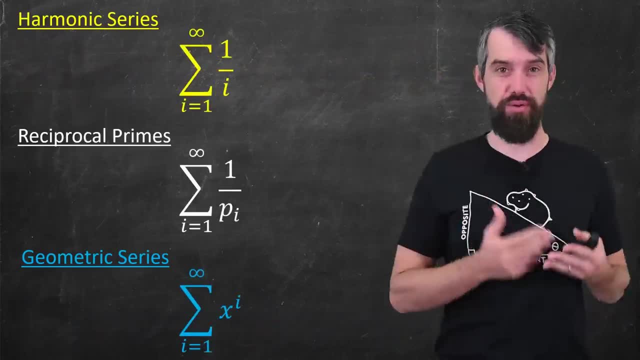 harmonic series that diverges, the geometric series that converges, and we don't know where those reciprocal primes are going to land. I can clean up my long expansions with summation notation, where here by pi I mean the i-th prime number and for the geometric series. 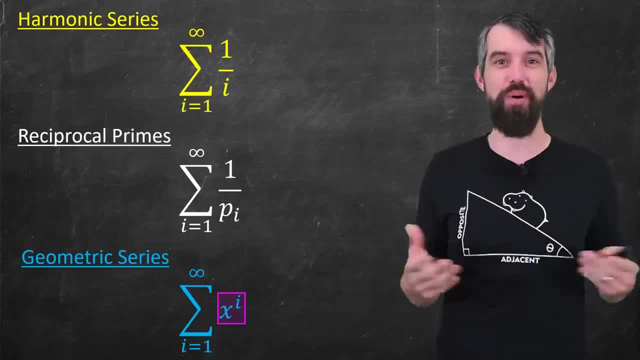 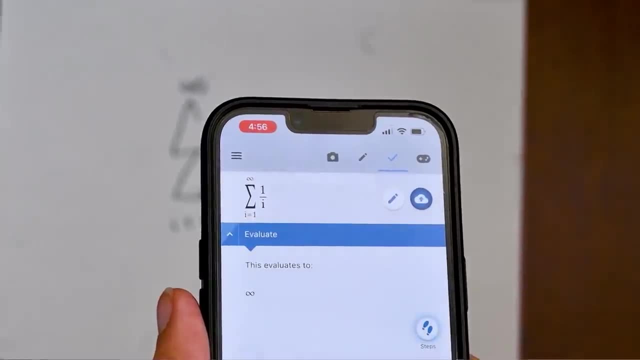 I had previously used x equal to one-half, but I can talk about it a little bit more generally. Let's input the harmonic series into Maple Calculator and we can see that the calculator shows us that it does diverge. But what I find interesting is that 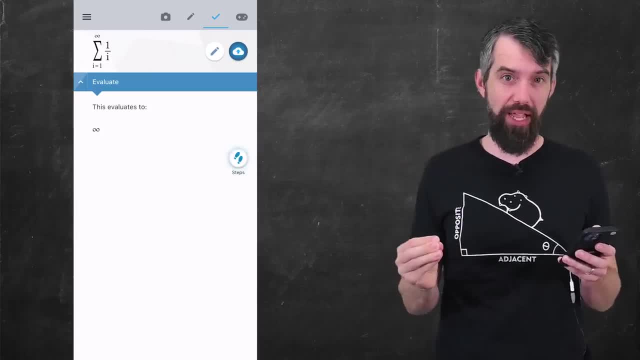 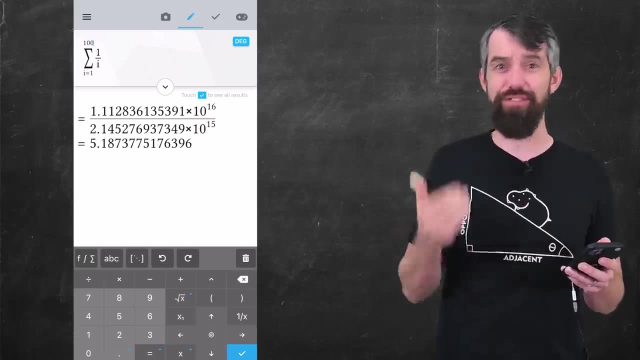 it actually diverges really, really slowly. For example, if I plug in one-hundred for the upper bound, as opposed to infinity, it's only a number like five. And if I went even further and put in like a million, this only adds up to fourteen. 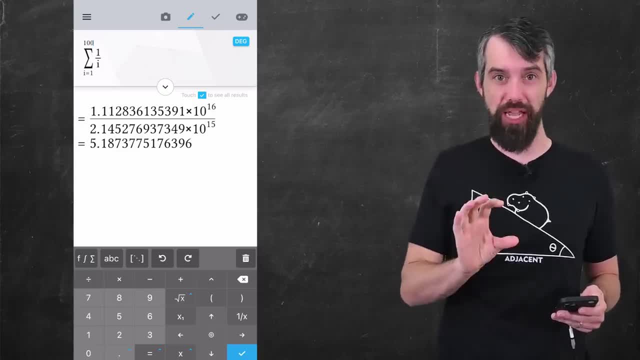 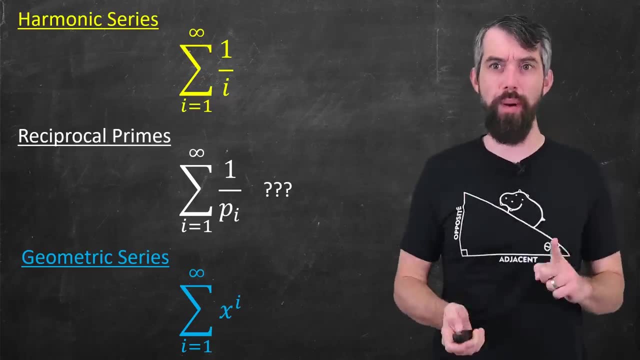 The harmonic series diverges, but it diverges slowly. My thanks to Maple Calculator for sponsoring today's video. more about them at the end. All right, so reciprocal primes. we don't know about harmonic series, we know diverges. and for the geometric series, 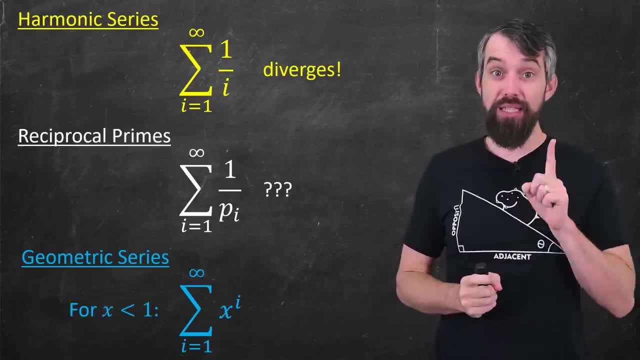 I can actually see that it diverges really, really slowly. So let's say more. when it converges, Namely if x is less than one, then this converges to one over one minus x. I know the value that it converges to. 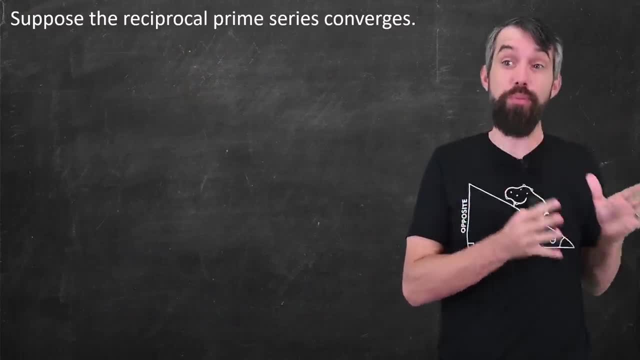 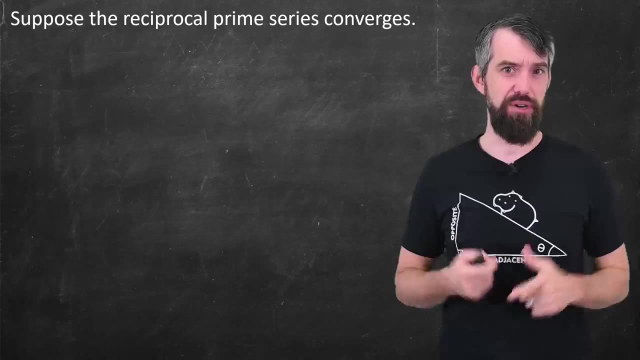 So let's begin our proof. Let's start with the assumption that the reciprocal prime series actually converges, And I'm going to argue by contradiction. If it converges, let's say it converges to I don't know a million. 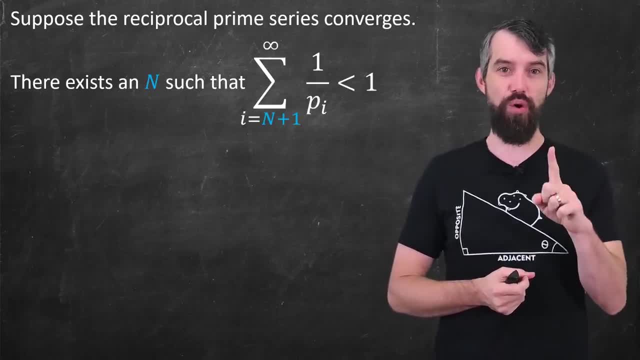 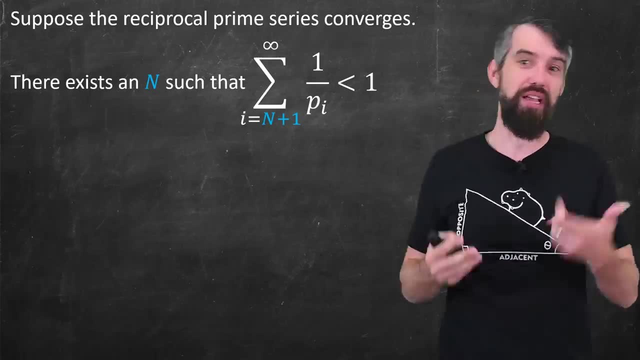 then at some point there is a value n, where the terms from n plus one all the way to infinity are smaller than the number one, Like, for example: suppose the sum of the reciprocal primes converges to a hundred. just to make up an example. 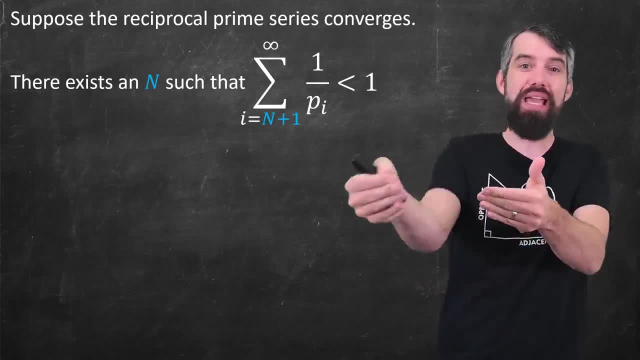 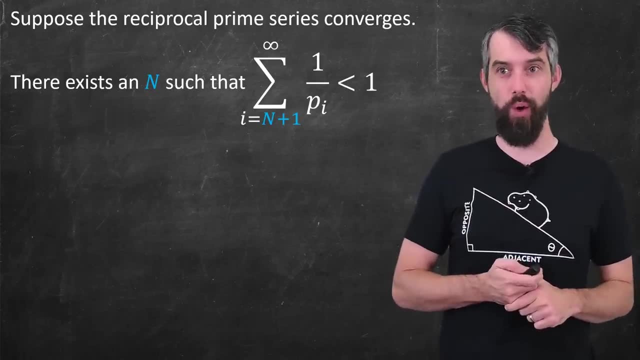 Then at some point you would have gotten to ninety-nine and all the remaining terms would be the ones that were less than one. So, regardless, we have some value of n, where this series is less than one, and whatever that number is some number less than one. I'm just going to give it a name. 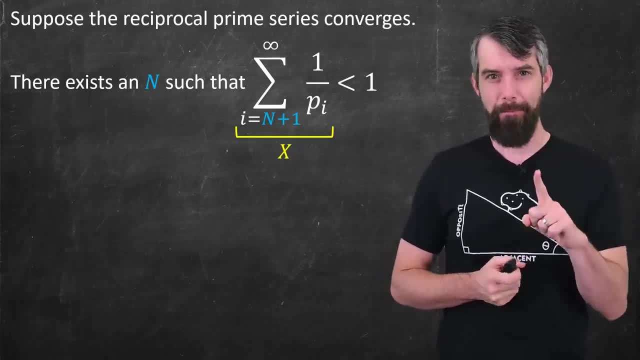 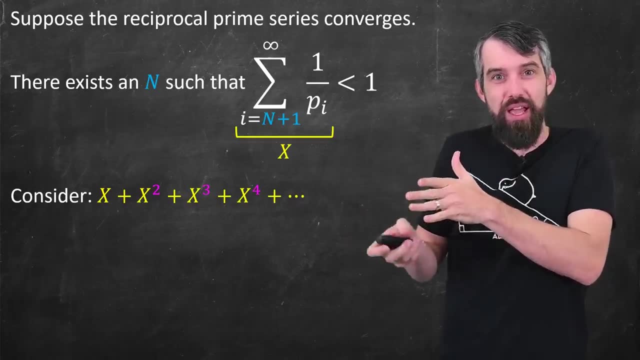 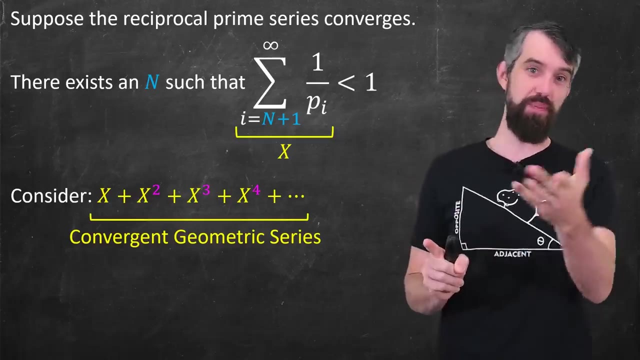 I'm going to call it x, Okay. So now let me make a new series for you. Consider the series x plus x squared, plus x cubed, plus x. fourth. This is a geometric series And it's a geometric series that is, a convergent geometric series, because the value of x was 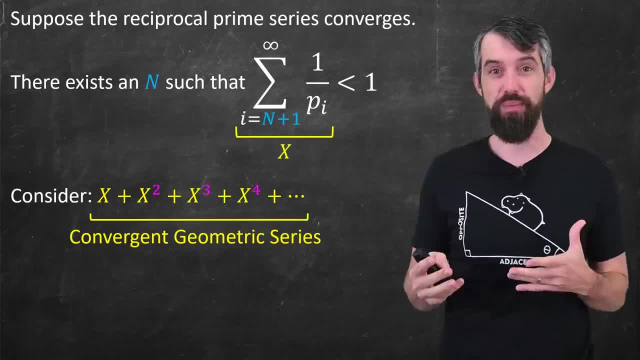 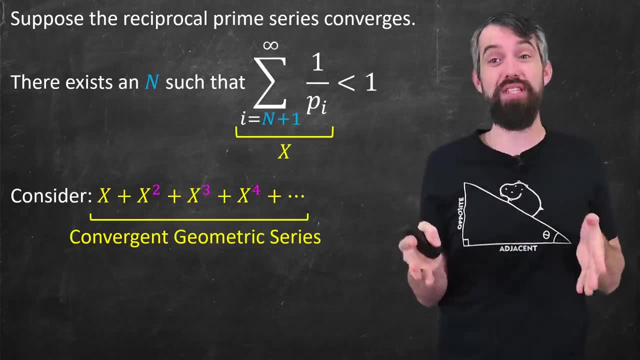 less than one, which we had just argued meant that the series would converge. It's a strange series Like each of these x's is itself this infinite series, And then I'm taking powers of those x's and making a new series out of that. 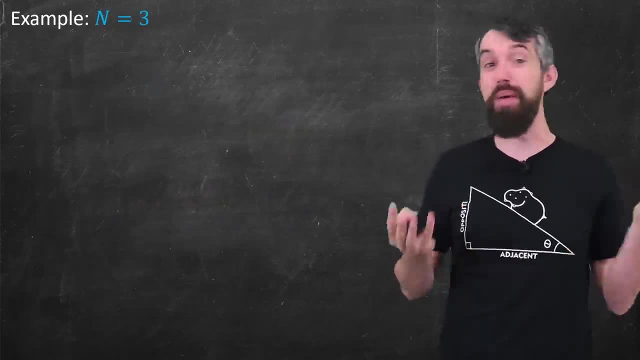 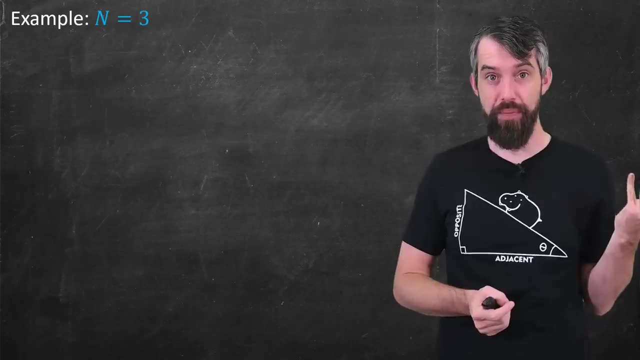 Just as an example, Imagine n was three. It's probably not, It's probably way bigger than that, But suppose it was three. So that would mean two, three and five, the first three prime numbers we're going to throw out. 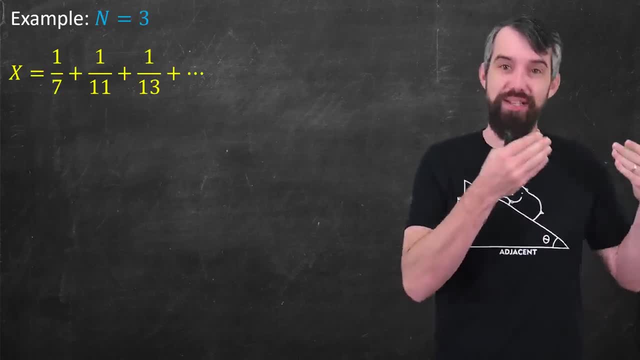 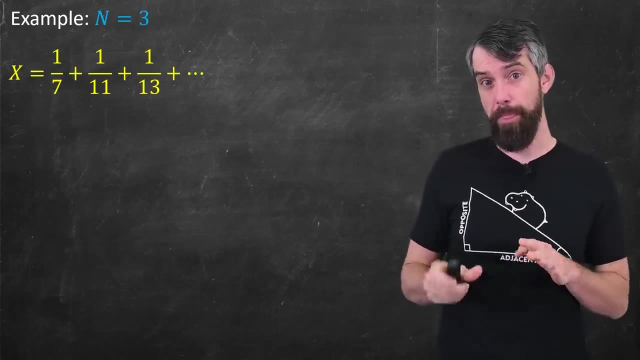 And then I'm just going to consider my sum x to be things like one seventh, one eleventh, one thirteenth and so on, All of those reciprocal primes, not including the first three. Okay, So now let's take a look at what our geometric series is, where we take powers. 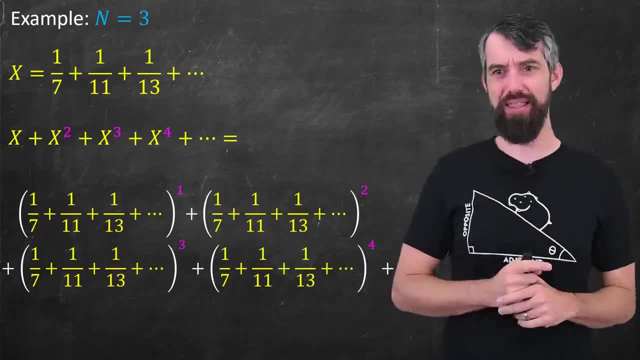 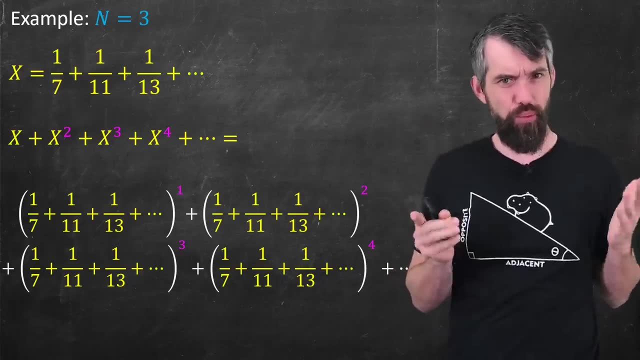 Well, it's going to be long and messy, so we'll put something up like this and I'll include that dot, dot, dot And every one of those bracketed expressions that we raised to a power. So this is a very weird object and I want to try to understand, like what things are. 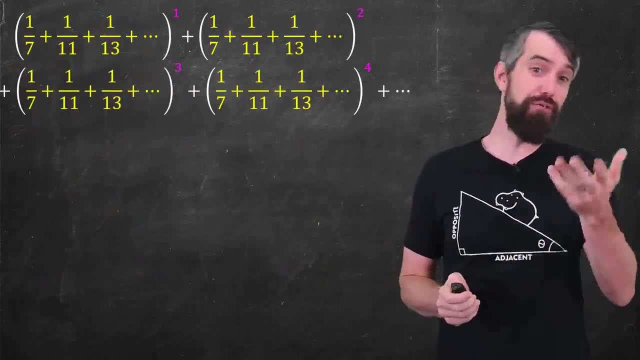 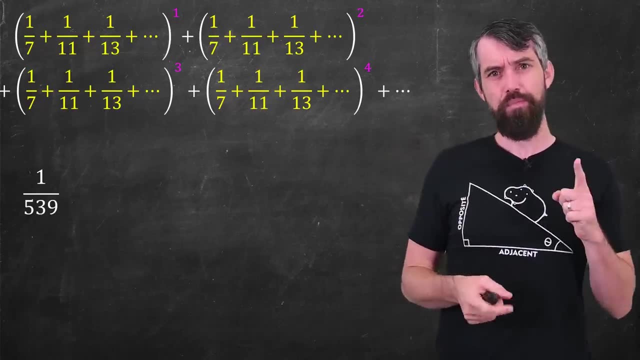 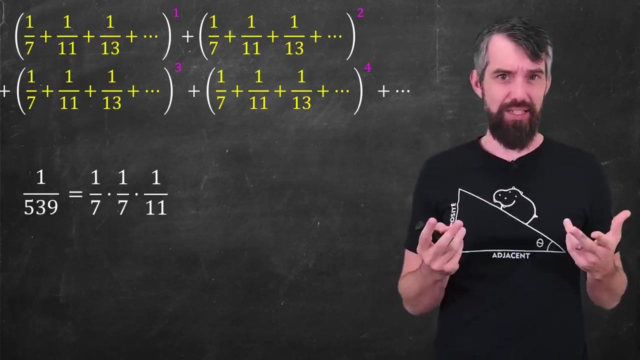 actually inside of this particular object. For example, take the number one over 539.. Is that in this series somewhere? Well, 539 has a prime factorization of seven times seven times 11,, that is, it's three primes multiplied together. 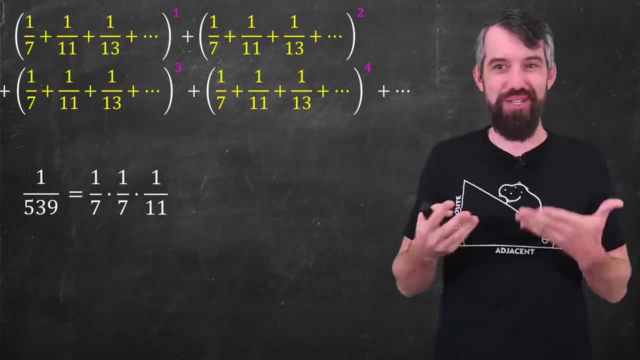 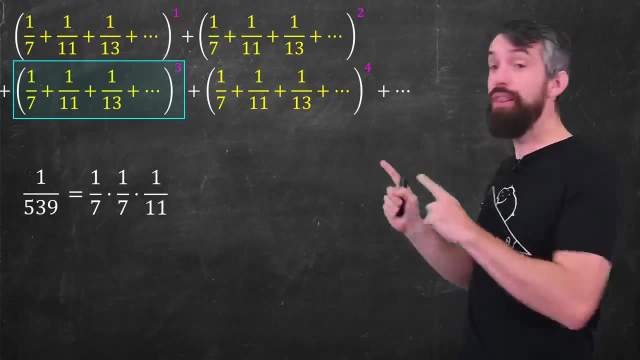 Okay, So the numbers are over the threshold that we talked about. They're all one seventh or larger, So that number of one over 539 occurs somewhere in this expansion- the cubed expansion here, where you're choosing three different numbers and multiplying them together. 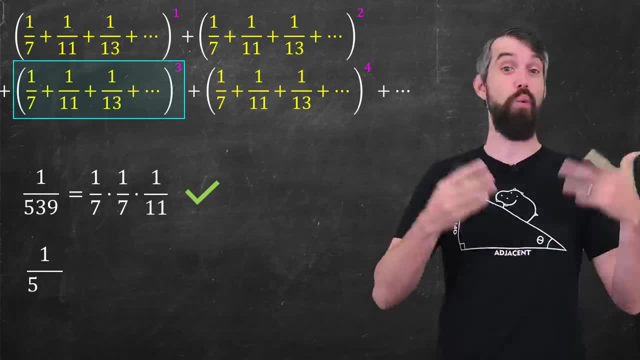 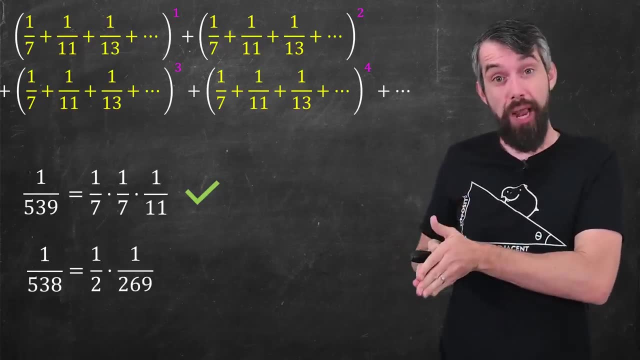 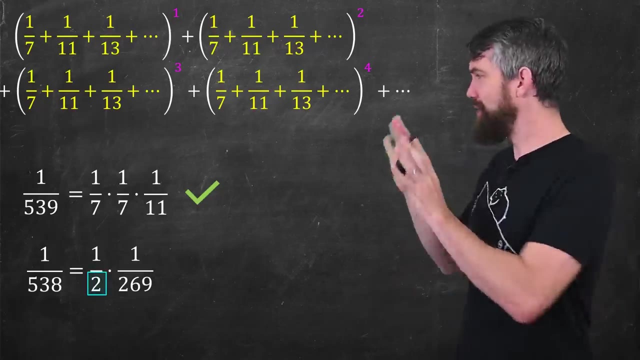 So yes, one over 539 is in the expansion. Okay, What about one over 538 then? Well, the prime factorization of 538 is two times 269, 269 is a prime number. It's somewhere in the dot dot dots there, but there's nowhere where this one half factor. 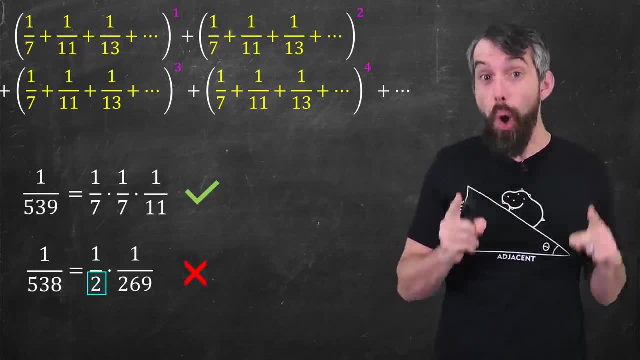 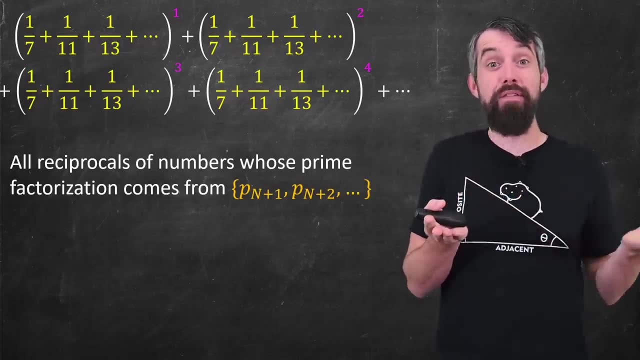 is ever going to occur. So 538 is not in that expansion. That is, what I'm really considering is the reciprocals of all numbers, where, when you take their prime factorizations, all of those factors come from the n plus one prime, the. 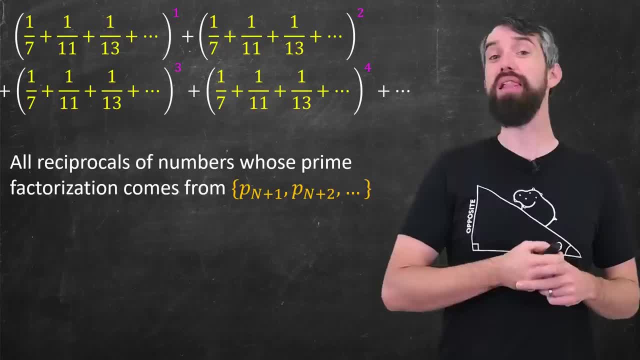 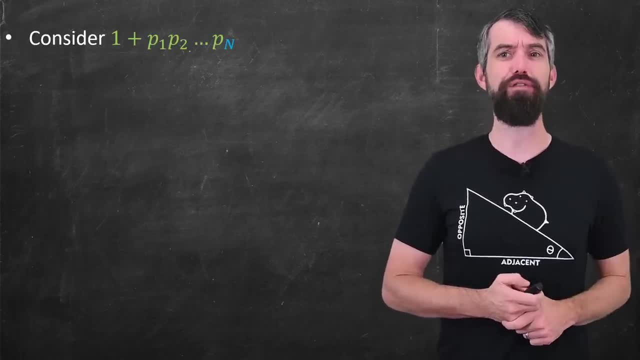 n plus two prime and so forth. Okay, So a lovely property, not yet clear how this is going to help us. Next thing I want to talk about, I want you to consider the following expression: one plus the product of all of the primes. 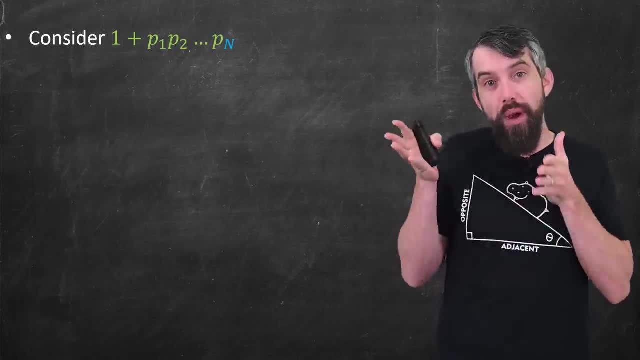 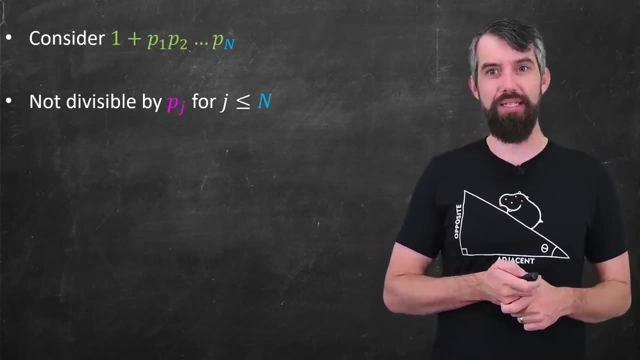 the first prime, which is two, the second prime, which is three, all the way to the nth prime. This is a kind of funny object. The first thing I want to note is that it is not divisible by any of the primes less. 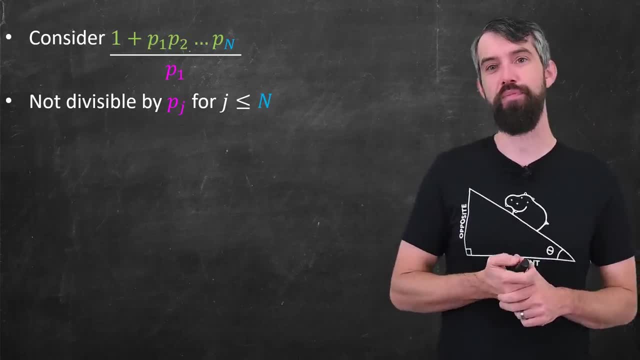 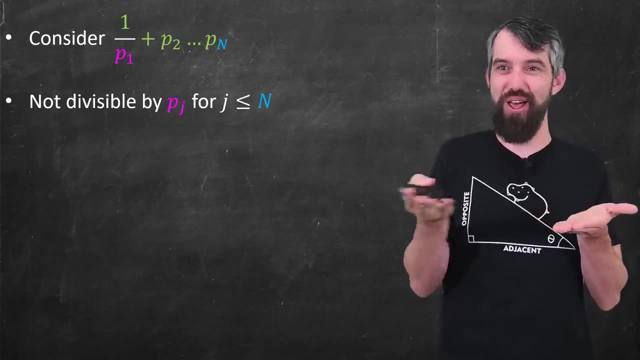 than n. Let me just try to divide out by I don't know. say the first prime, p1. Well, at the front I would just get one over p1. And then the p1 would cancel the p1 in the expression that has a lot of primes multiplied. 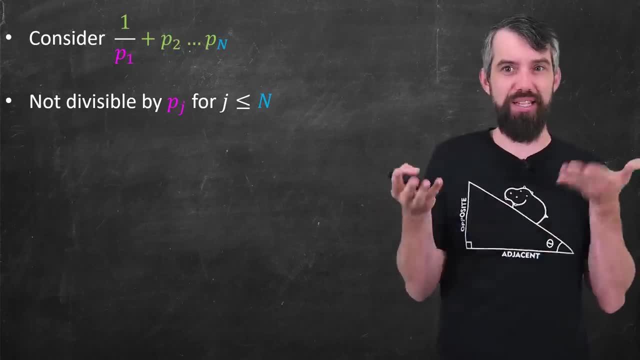 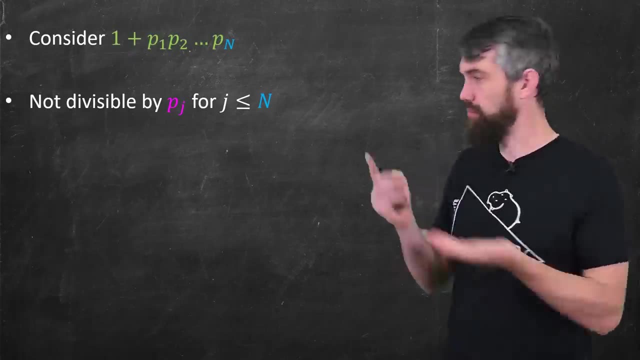 You'd be left with p2 down to pn. P2 to pn is an integer, but one over p1 is not an integer. This is not an integer. It's not divisible by p1.. Okay, So let's return to the expression. 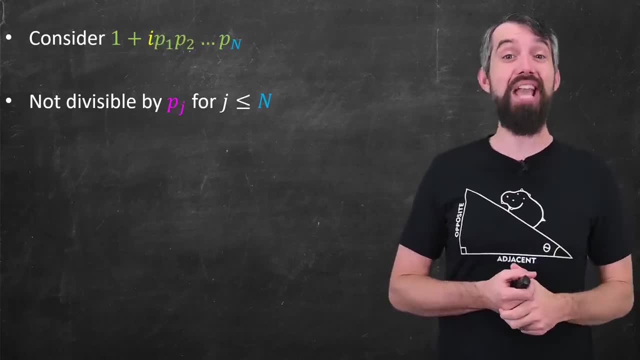 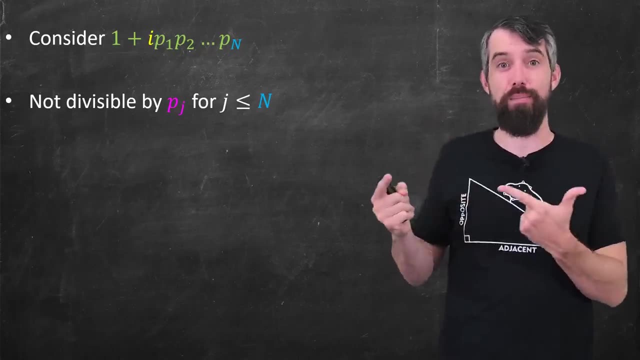 And actually this is true if I then multiply an i out the front, If I put any multiple of that p1 down to pn, it's just not divisible by any of the first n primes. By the way, If you've seen my video proving that there's infinitely many prime numbers, you can go. 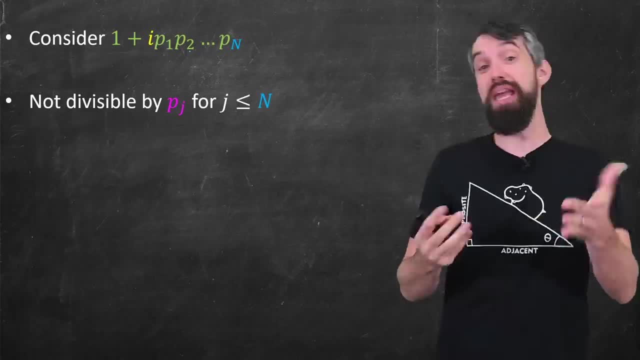 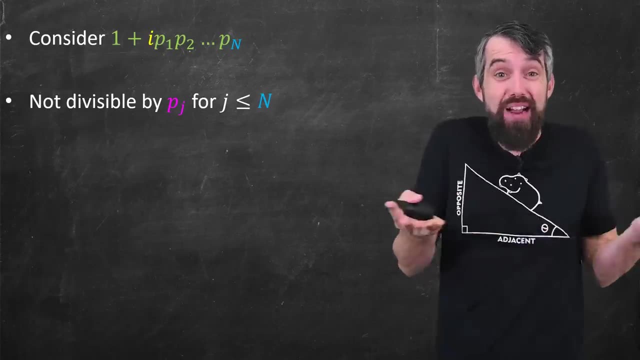 and check that out, then you'll notice that this basic expression is one that we had to use in that video as well. So this is kind of returning to us. Regardless, what this means is if I try to figure out what is the prime factorization. 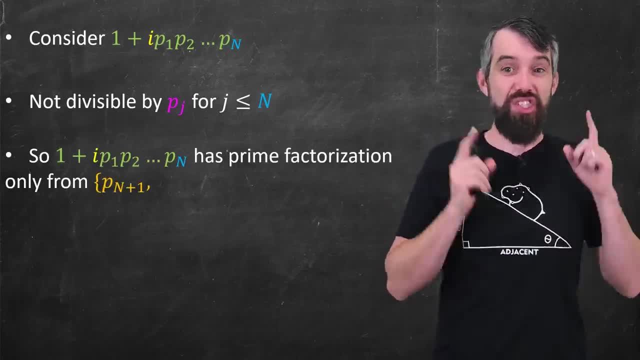 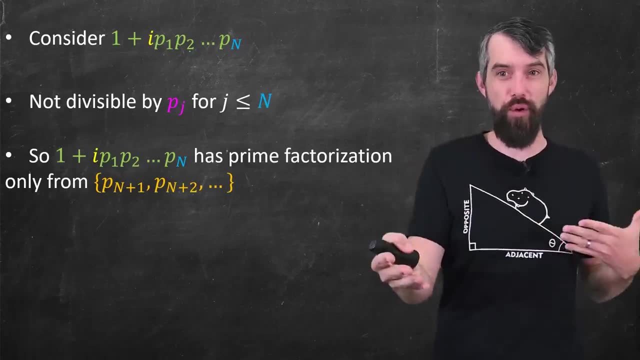 of one plus i p1 down to pn. Well, that is something like the things we were just talking about, Something coming from the n plus first prime, the n plus second prime, and so forth. One plus i p1 down to pn. 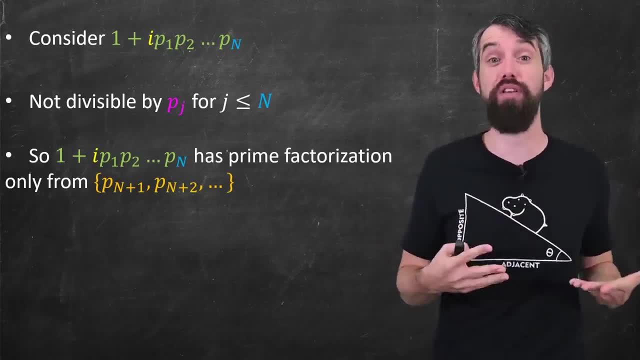 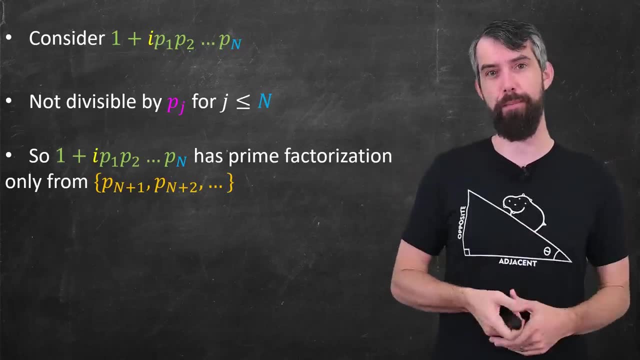 Has no prime factors in it that are less than n, so all of them must be more than n. Okay, so I think I've collected all the random tools that we're going to need in our proof, so let's put them all together. 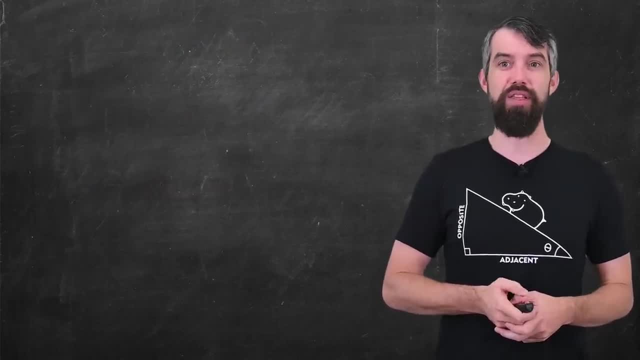 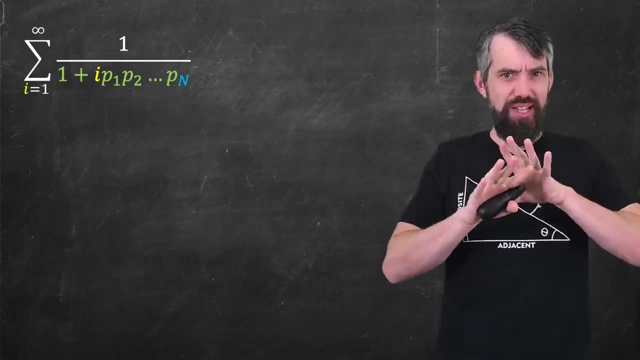 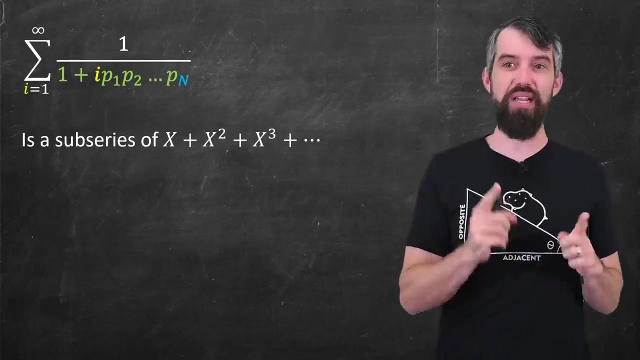 I want you to consider the following new series. This is the sum, from one to infinity, of one over one plus i p1 down to pn One over those expressions that I was just talking about. My claim is that this series is a sub-series of the x plus the x squared. 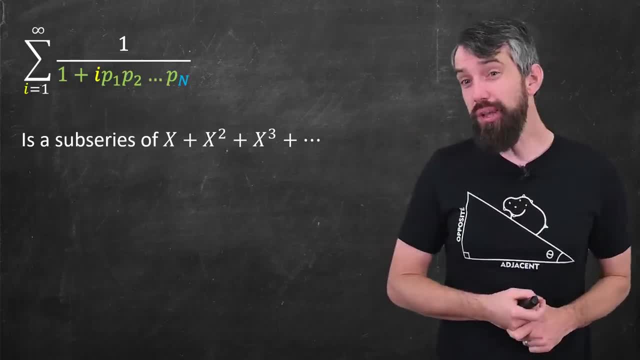 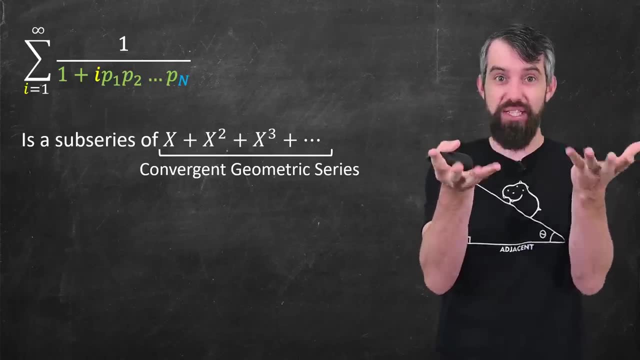 Plus the x cubed that we were talking about, Which we had argued was a convergent geometric series. What do I mean by a sub-series? Well, all the terms in the sub-series occur in the main series, but the main series might have even more terms. 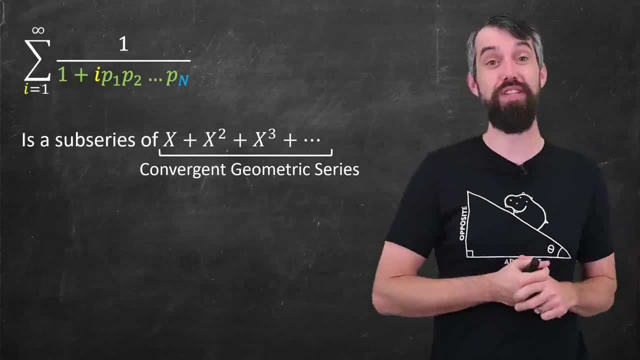 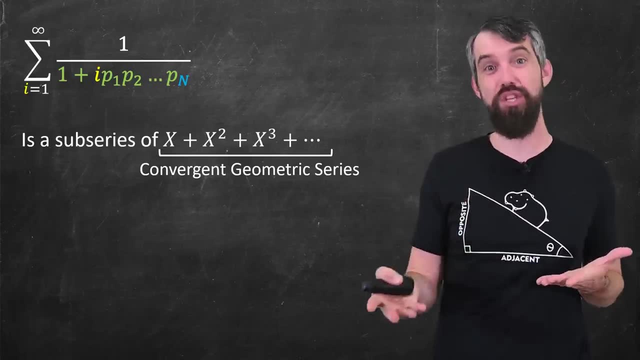 And indeed, what we had just spent all our time arguing was that our denominators of this series looked like the type of the objects that were in the geometric series, The x plus x squared plus x cubed series, So indeed, everything in this new series I'm talking about. 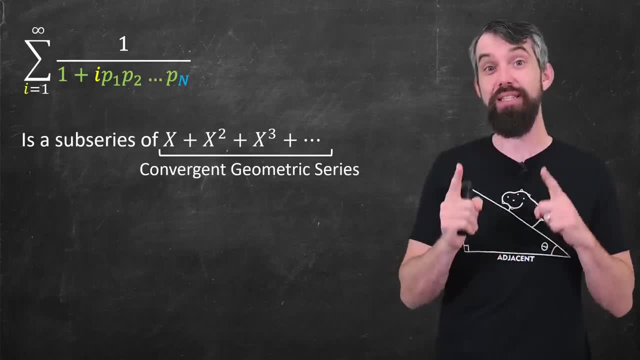 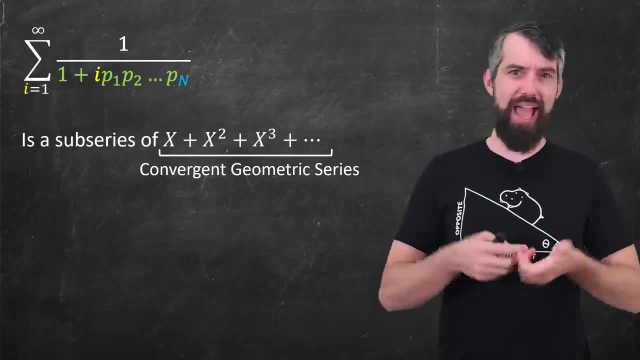 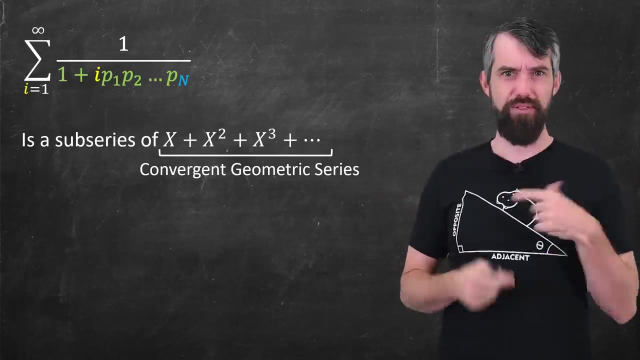 Would have shown up in the geometric series. This is a sub-series, Okay, so let's analyze that sub-series. When I look at this, I think when n gets really large, the plus one is not going to really matter. When I look at the p1 down to the pn, that's just a constant multiplying by the i. 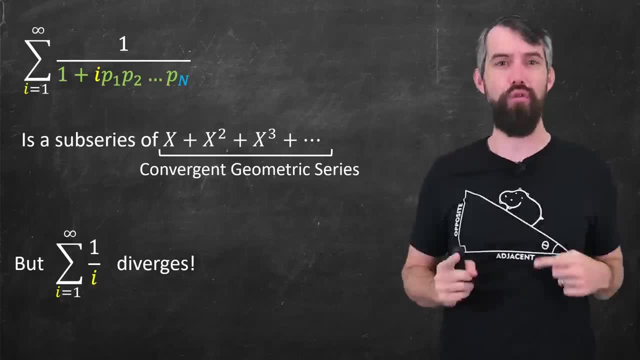 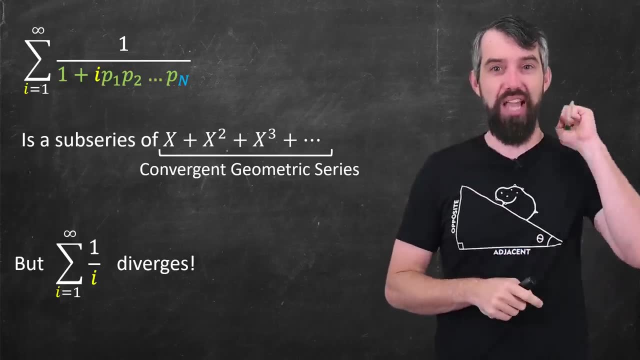 So when I look at this heuristically, I just see one over i. The constants I sort of know are not going to matter, and I'll be precise about this in a moment. When I look at the top series, it looks like a harmonic series. 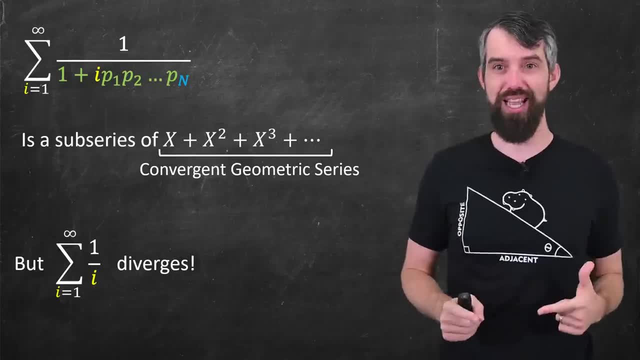 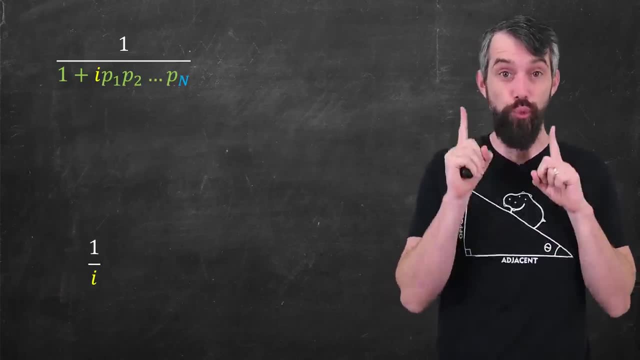 Okay, let me be a little bit more precise about how I can compare this more complicated one on the top to the harmonic series. If I just consider the terms, let me consider their ratio and I'm going to do something called the limit comparison test from calculus. 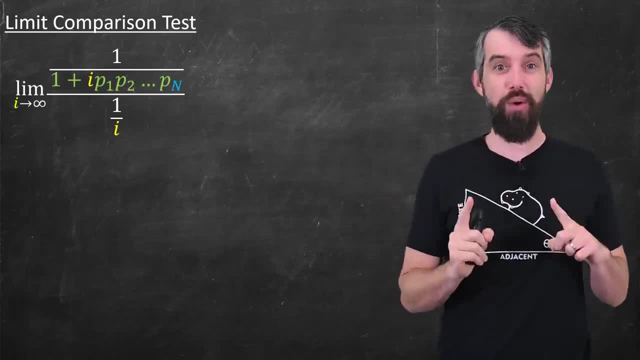 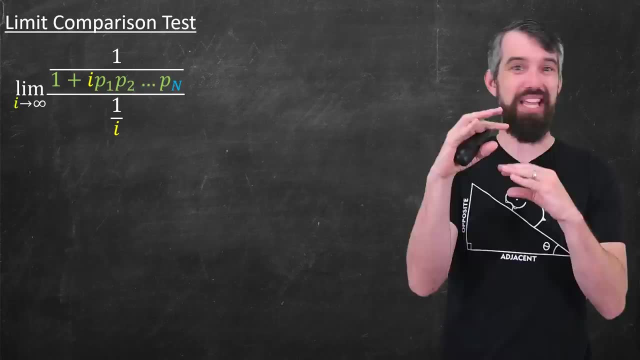 I have a video on that you can check out if you're so interested. And basically what I'm saying is if I look at the ratio of the terms in my series, if one goes to infinity and the other is just like a constant multiple of that, it's going. 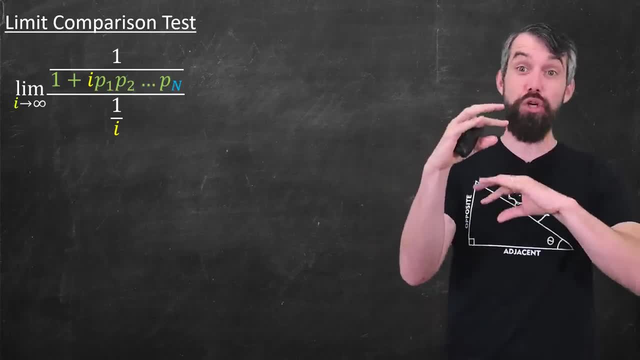 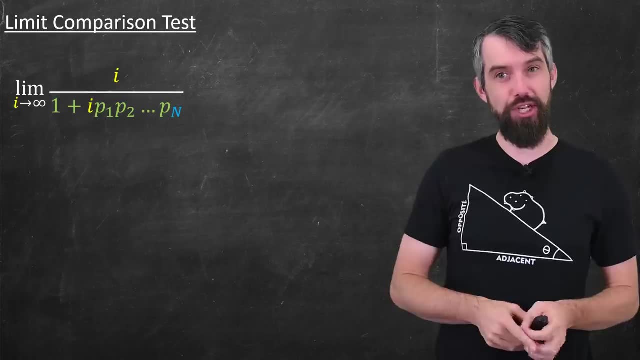 to be dragged to infinity as well. So I'm going to look at the ratio of the terms. as i is going to go to infinity, I'll bring the one over i up and combine it into a simpler expression And then, as the i goes to infinity, taking that limit, it's just one over p1 to pn. 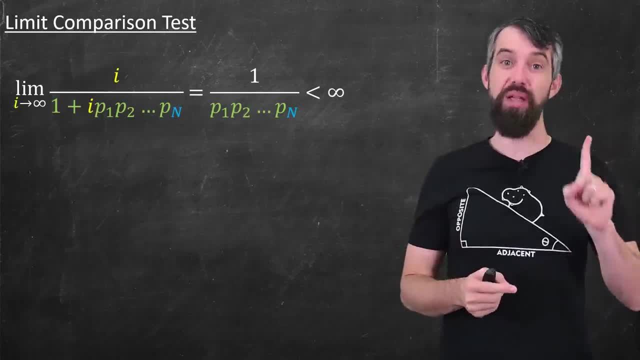 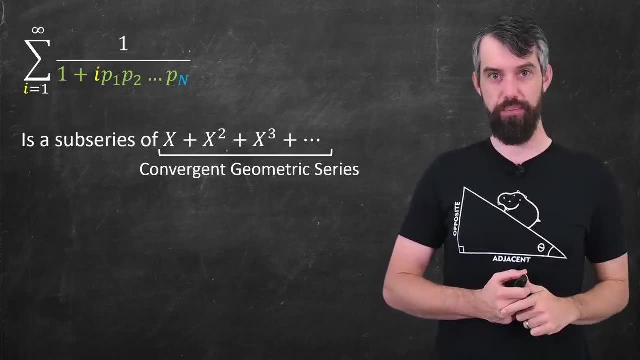 It's a number, It's a finite number, And so the limit comparison test works, And indeed we can say that the series on the top behaves like a harmonic series. A harmonic series, we know, diverges, And this gives us a contradiction.